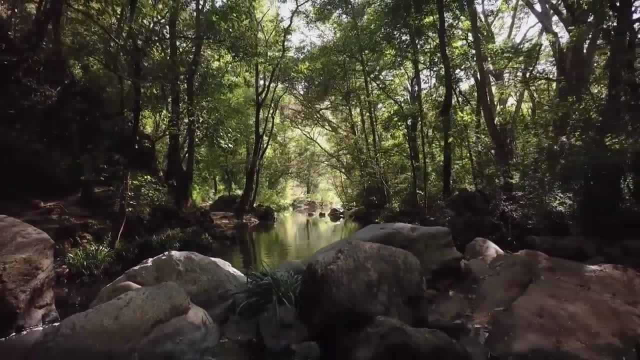 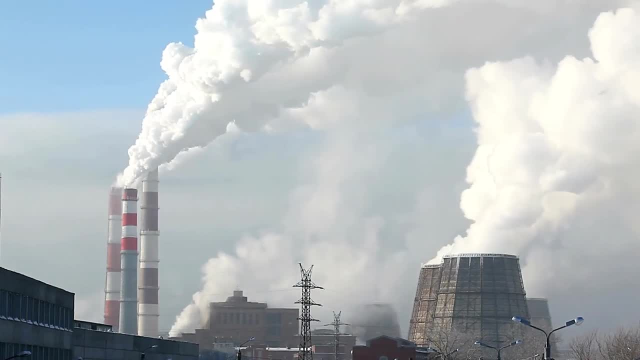 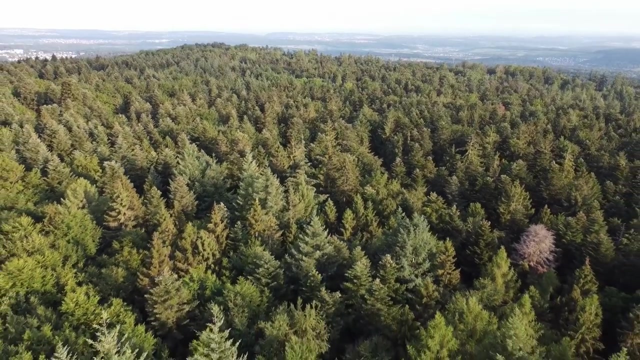 radioactive waste, improper resource utilization, deforestation and many other environmental issues. After identifying and analyzing these issues, they design and develop the appropriate solutions that meet sustainability standards. This may involve the use of innovative technologies or working with legislators and other stakeholders to develop sustainable policies. So, in a nutshell, 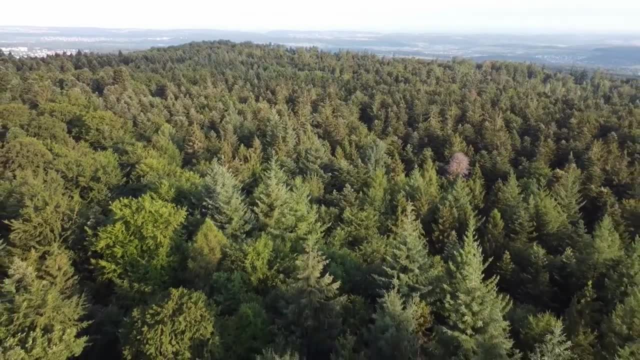 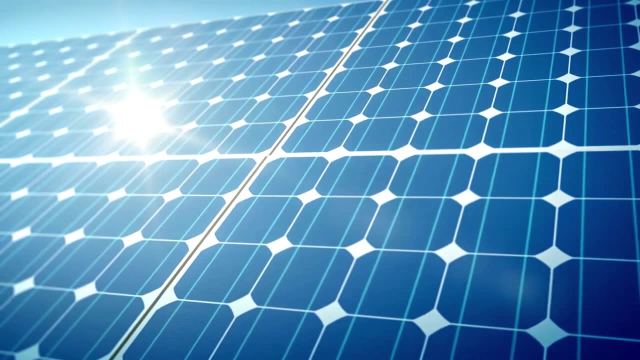 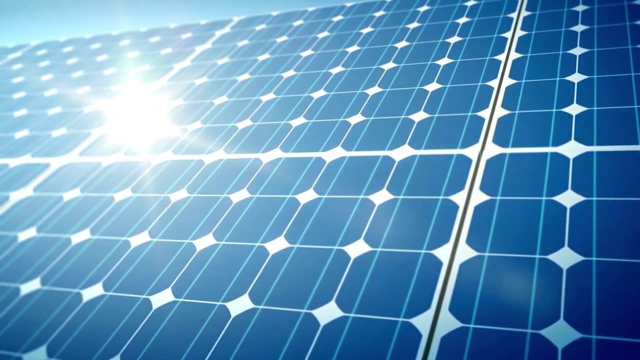 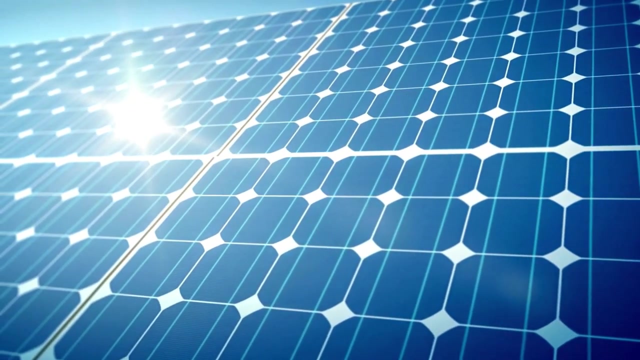 environmental engineers assess, analyze and mitigate the impact of human activities on the environment. The specific duties of environmental engineers are based on the industry in which they work. For instance, the duties of an engineer in the agricultural field may include assessing the impacts of agricultural practices on water and soil quality. However, the duties of an engineer within the manufacturing field may involve creating processes that reduce the manufacturing process. The duties of an engineer within the manufacturing field may involve creating processes that reduce the manufacturing process. The duties of an engineer within the manufacturing field may include creating processes that reduce the manufacturing process. профiles andyer. 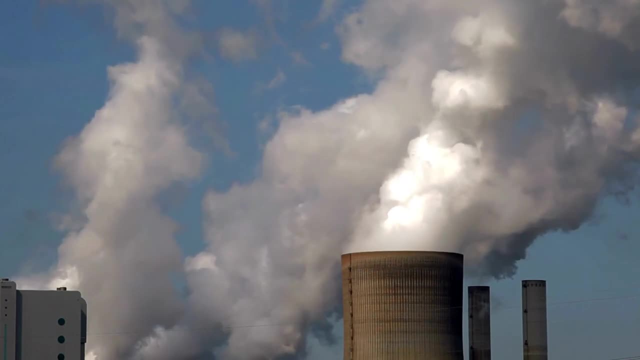 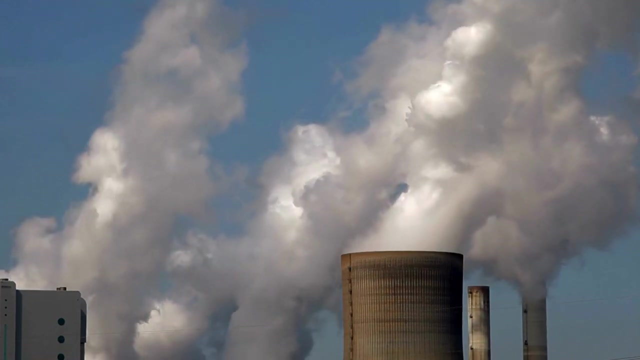 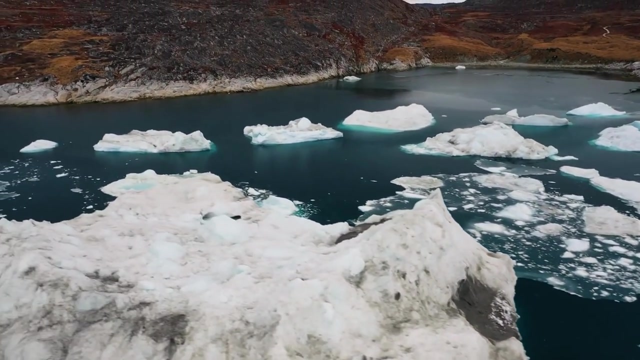 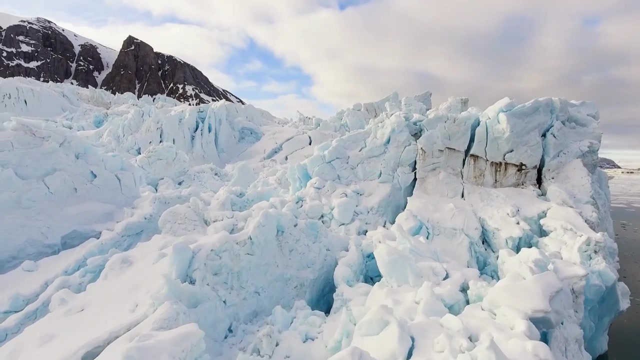 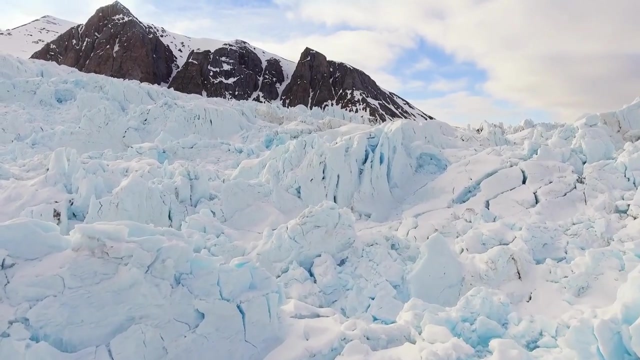 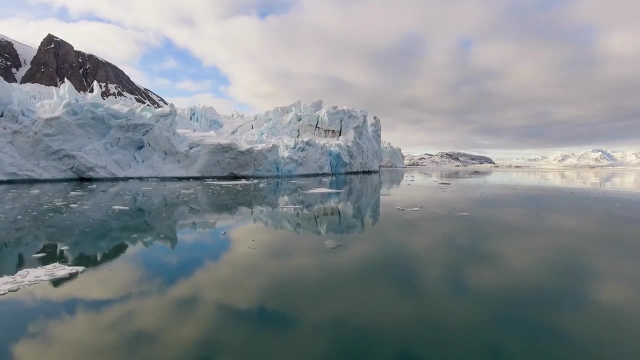 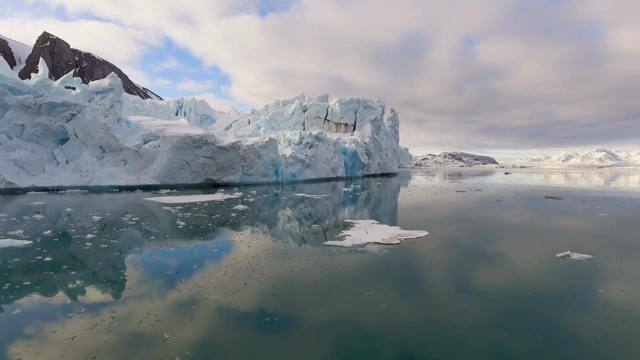 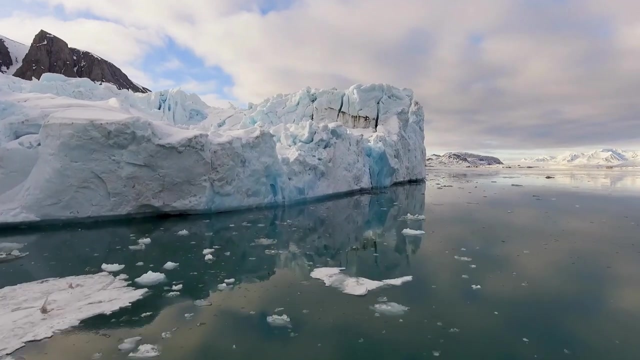 skipping to transition fromijkb. The work is all geared towards maintaining and promoting environmental health and safety. For example, one important aspect of this role involves creating and reviewing environmental reports to identify potential areas of concern. Ensuring that organizations are compliant with standard operating procedures, best practices and legislation is also a crucial part of this role. 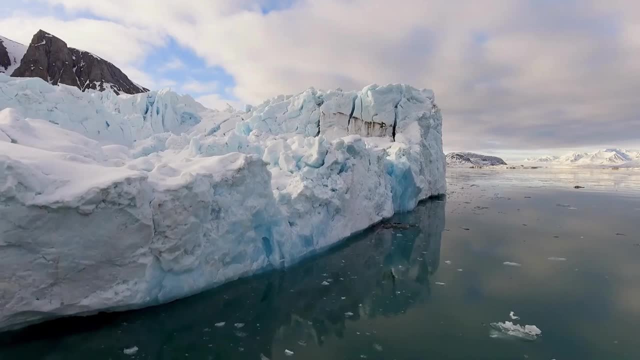 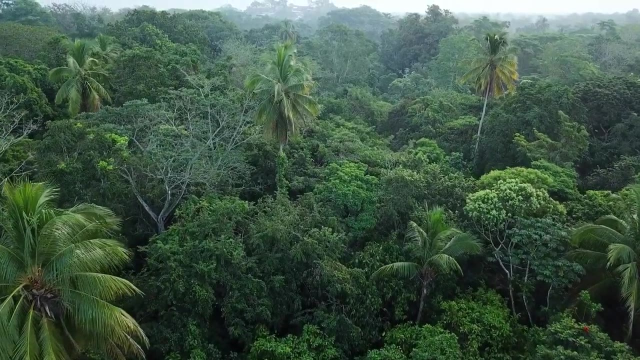 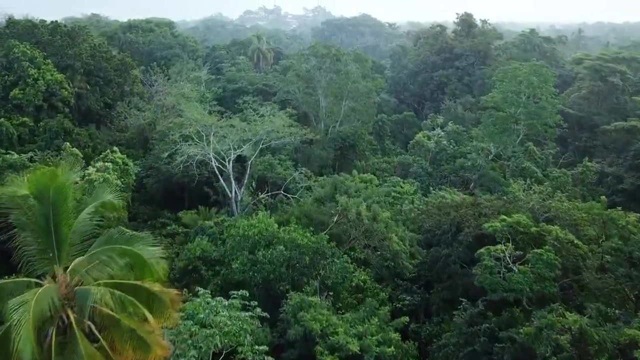 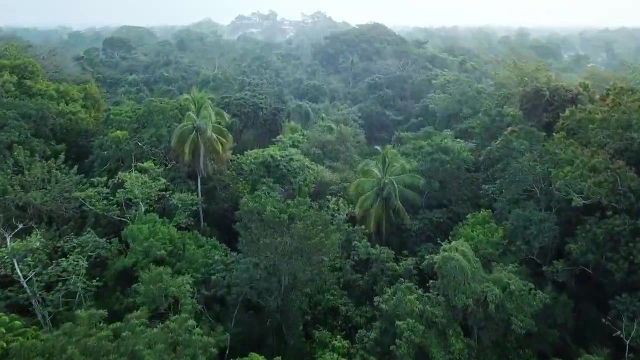 Additionally, environmental engineers often collaborate with governmental agencies and other stakeholders to improve existing or develop new regulations to address complex environmental challenges. Overall, the work of an environmental engineer involves a diverse range of tasks to promote and protect the health of the environment. The skills required to be an environmental engineer: 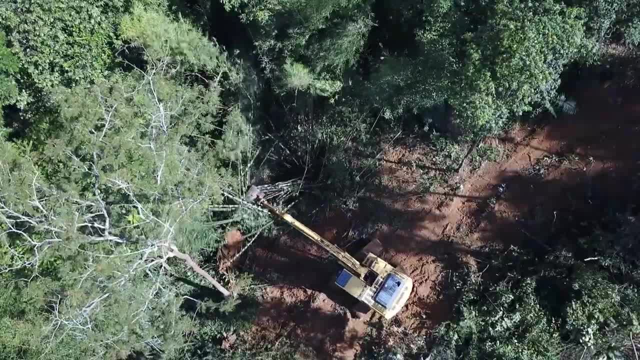 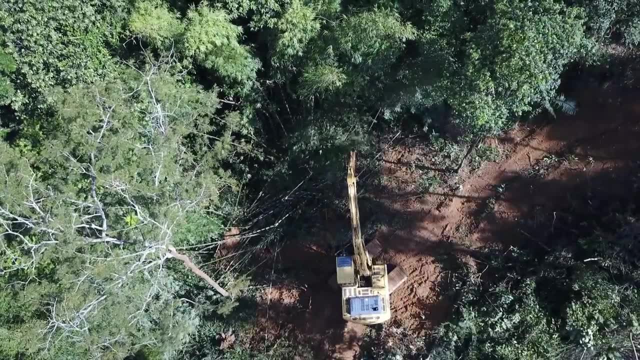 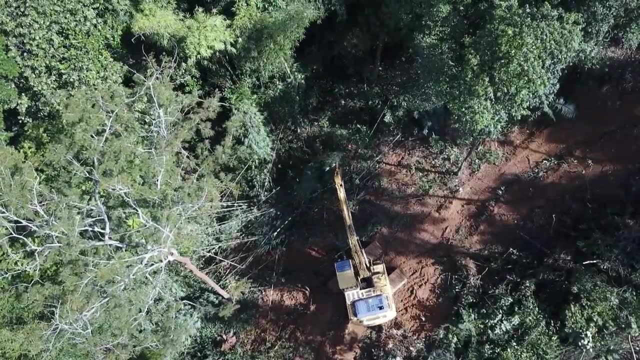 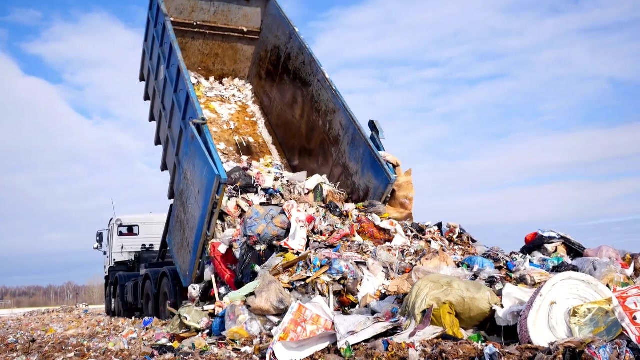 includes having strong problem-solving and analytical skills, because you must be able to assess and analyze issues that may arise and develop effective solutions to mitigate the impact to the environment. being detail-oriented, with an aptitude for collecting and analyzing scientific data. possessing effective written and oral communication skills. with the ability to work.